So I want to talk a little bit about what is a similarity ratio? all right, So here we've got an example of two triangles that are similar. How do I know they're similar? Remember the two things that have to be true: for any two polygons to be similar, The corresponding angles have to. 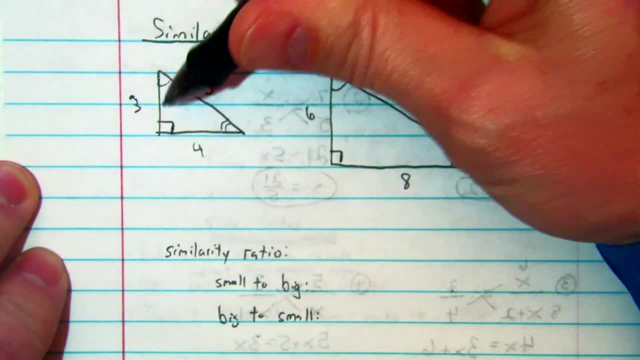 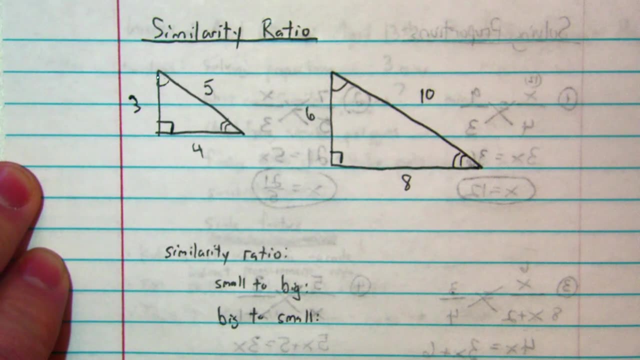 be congruent. So check this out: This angle is congruent to this angle. this angle is congruent to this angle because they're both right angles and this angle is congruent to this angle, So the corresponding angles are congruent. But also remember the second stipulation for triangles: to 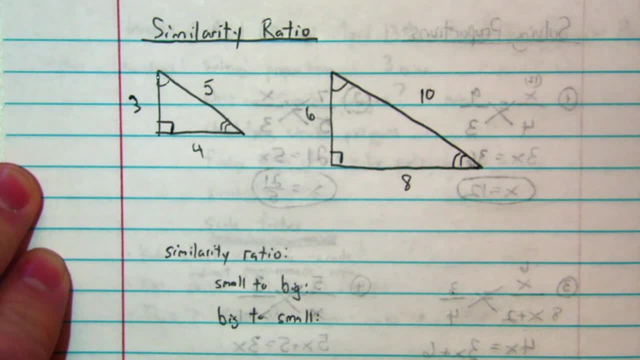 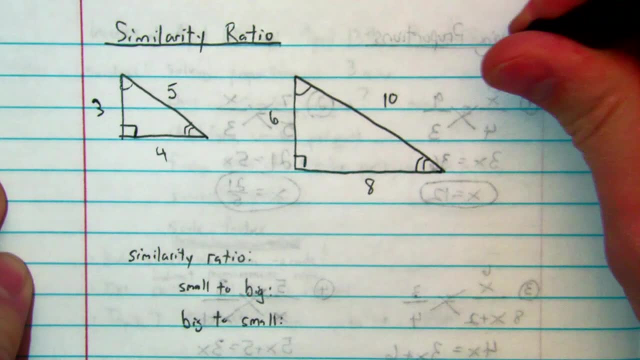 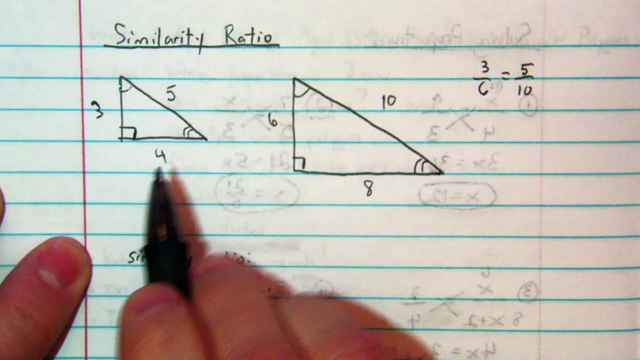 be similar is that the corresponding sides are in proportion. And we know these sides are in proportion because, if I write the fractions of corresponding sides, check it out: 3 over 6,, 5 over 10, and 4 over 8.. 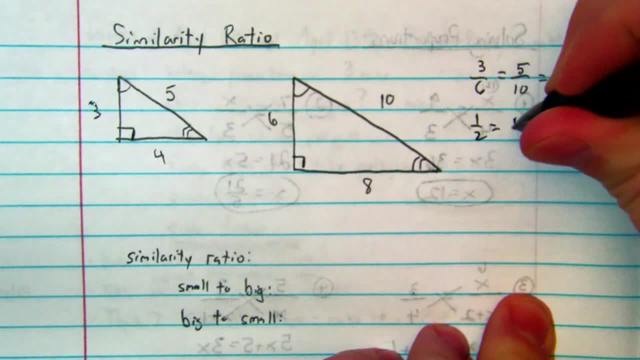 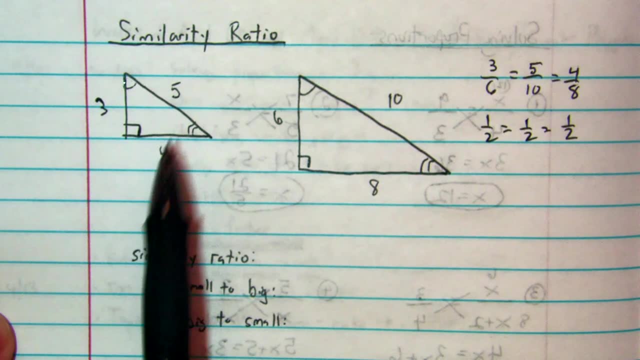 All of those fractions reduce to 1 over 10, and 4 over 8.. So now I know that the corresponding angles are congruent and the corresponding sides are in proportion, because all three of those fractions are equal. So if I want to talk about the similarity, 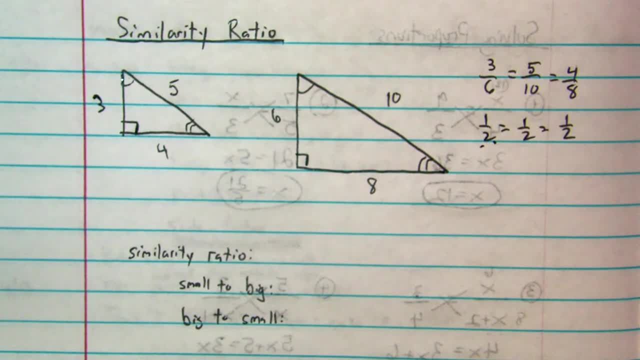 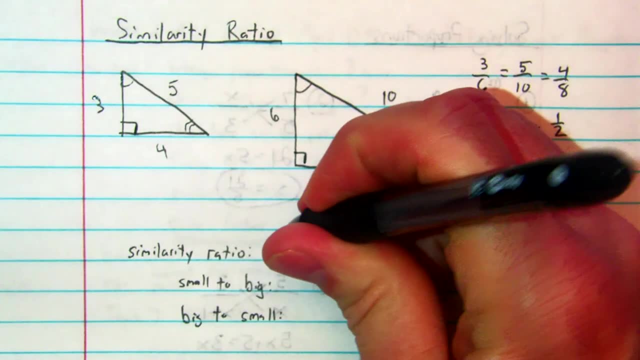 ratio. I mean this right there. that number is the similarity ratio. So I can write the similarity ratio one of two different ways. In this example right here I could say: the similarity ratio is 1: half. but that's saying, if I went from this triangle to this triangle, 1 to 2.. 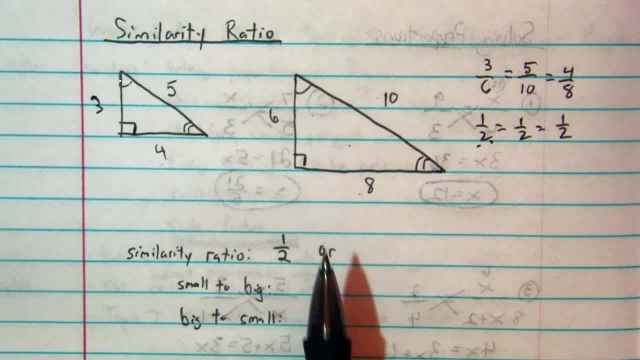 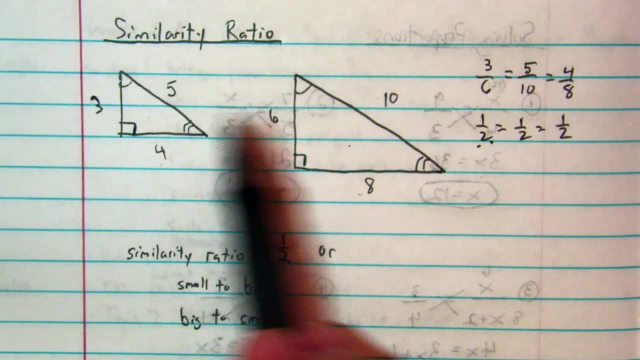 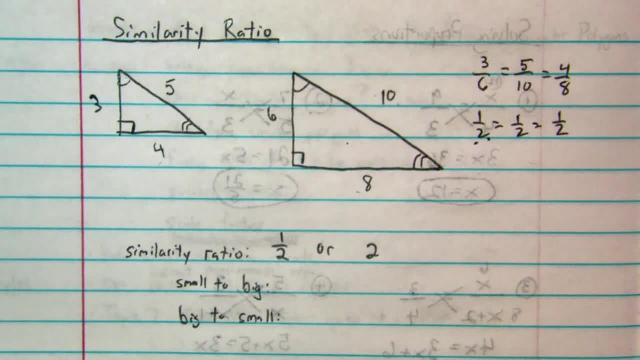 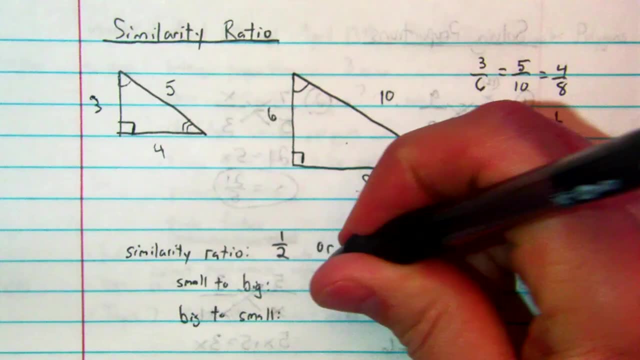 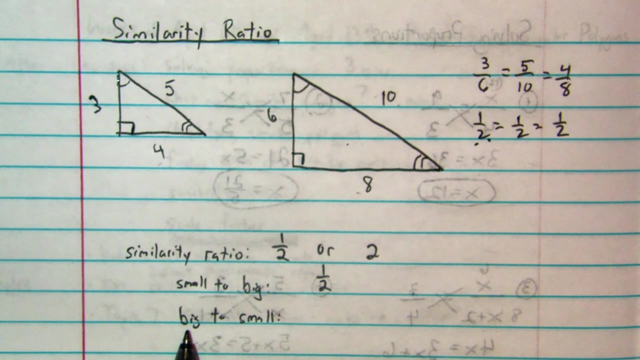 Sometimes the directions are going to be more specific, though. If the directions say to give the similarity ratio, in this case, from the small triangle to the big triangle, then you would say it's 1: half. If I asked you for the similarity ratio of the big triangle to the small triangle, then you would say: 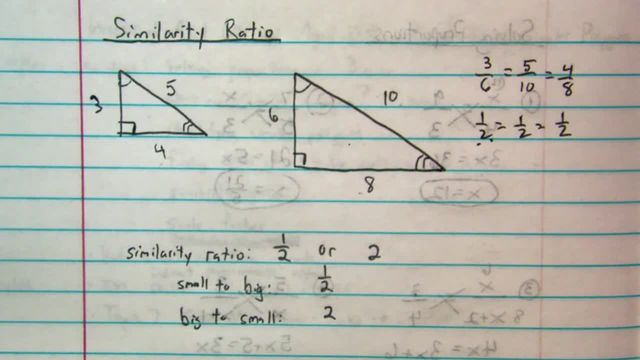 it's 2 to 1 or 2.. All right, So the similarity ratio is just the ratio of corresponding sides of two similar polygons. I hope that helps. Have a great day.